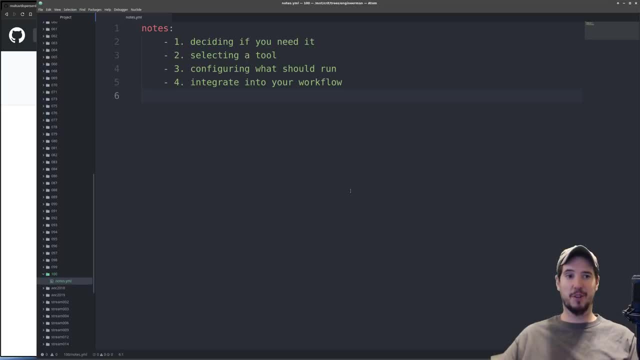 step, then it might be more effort to set up a continuous integration thing than it is to just do it manually. But if you're a group of developers working on the same code base and one developer over here writing a feature may affect another developer over here writing another. 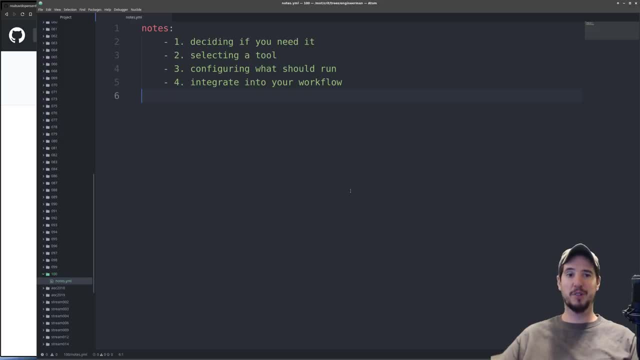 feature, then those are going to be the folks who are going to benefit the most by continuous integration, Because when both people push their features onto the shared branch and continuous integration automated test run, then you're going to find out right there if there's a problem, As 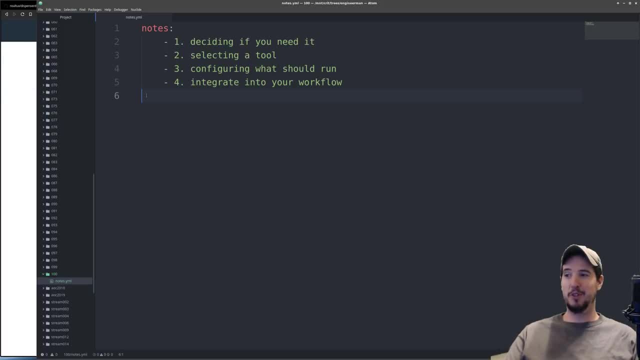 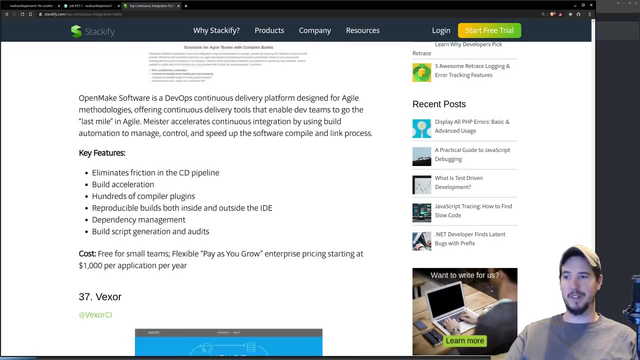 far as selecting a tool goes, it comes down to what features do you need and how much you want to pay. Now, with continuous integration tools, there are actually a million of them. There's so many, So there's not going to be any shortage of tools for you to choose from, And they're all. 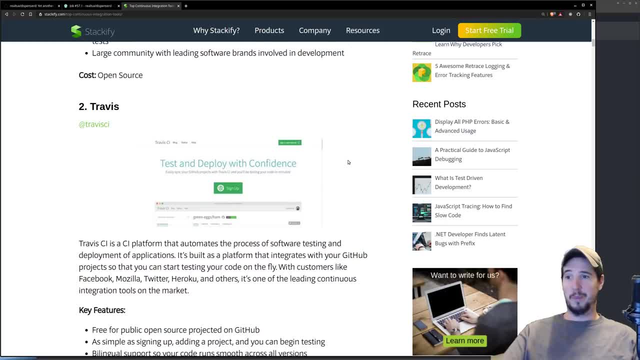 going to differ just based on feature set and cost. For all of our examples, we'll be using Travis CI just because the project that I authored several years back. Travis CI was the continuous integration product that I picked because at the time it was free for open source projects and I think it still is Worth mentioning. 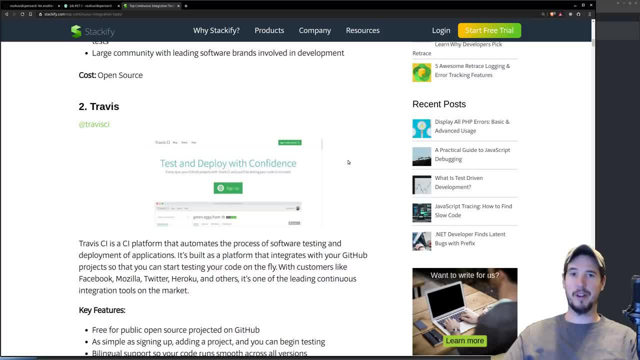 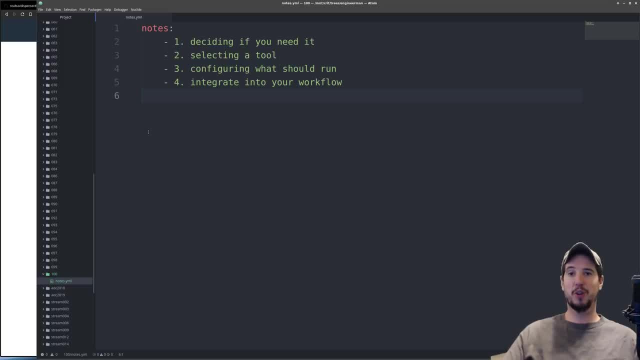 that I'm not being paid by Travis CI. it just happens to be the product that I used a while back. So now that we've decided that we do need continuous integration and that we've selected a tool, in this case, Travis CI- it's now time to configure exactly what should. 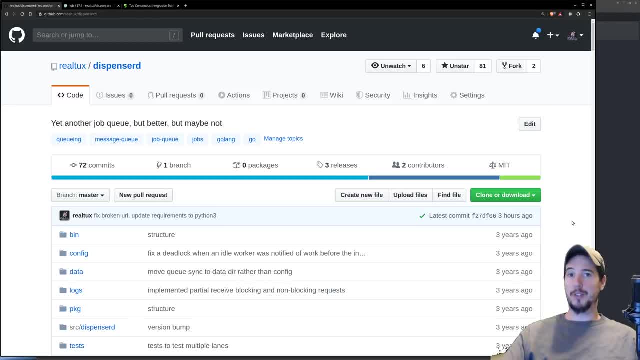 run. So to figure out that, we have to first look at the project. So this is a project I wrote a while back. It's called DispenserD. It's a go-to-configuration tool. It's a role-playing message queuing system that I wrote, purpose-built about five years ago. 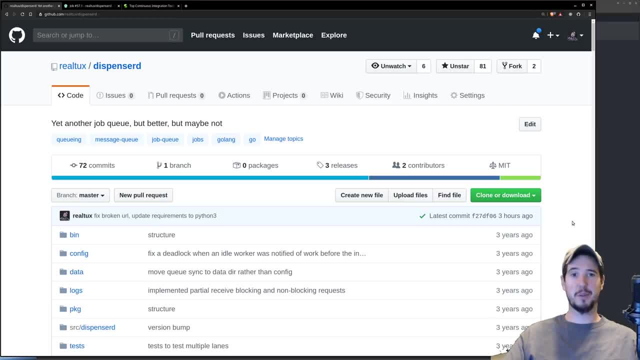 for an unrelated project. Now, what the project does is not necessarily important. However, this was an open source project that I did develop, that I did expect that people may contribute to and help me build. Additionally, because of the nature of the system being, 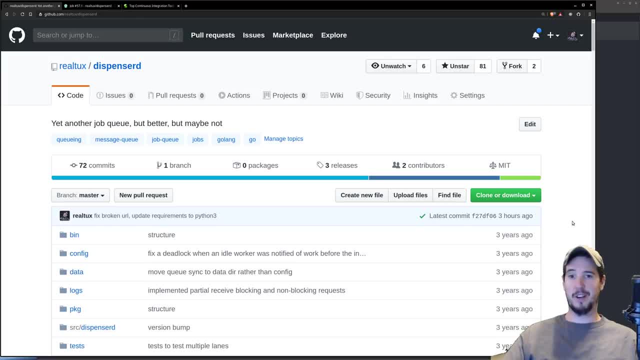 a message queue. it's important that the software absolutely does not fail, Otherwise it's going to cause chaos in people's projects. So because of those two facts alone, I knew I needed continuous integration and I knew I needed automated tests. 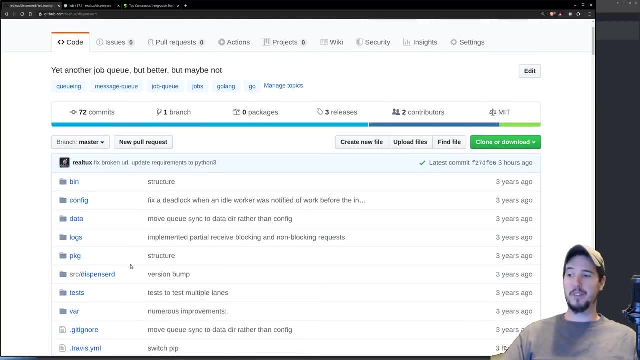 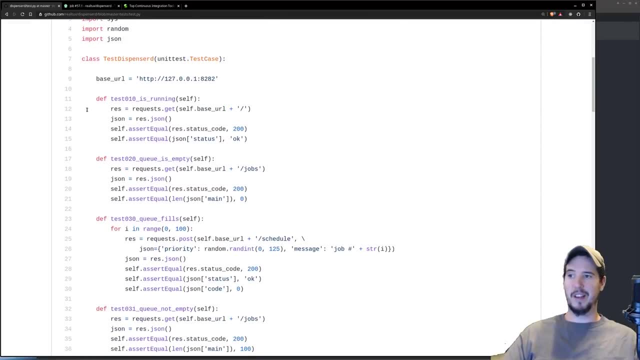 Now how to actually write tests. that's outside the scope of this video, but know that I have a folder called tests and in that folder I have a file called testpy and in that Python file I have a bunch of tests that are running against a running instance of. 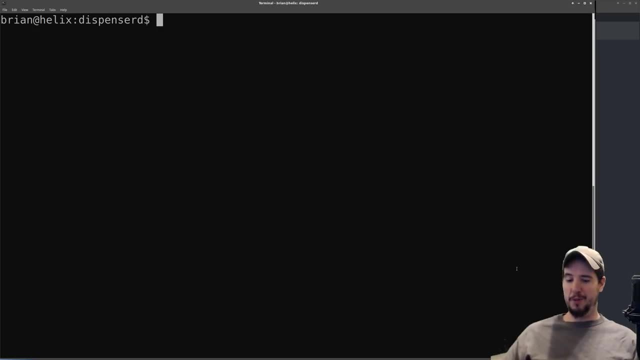 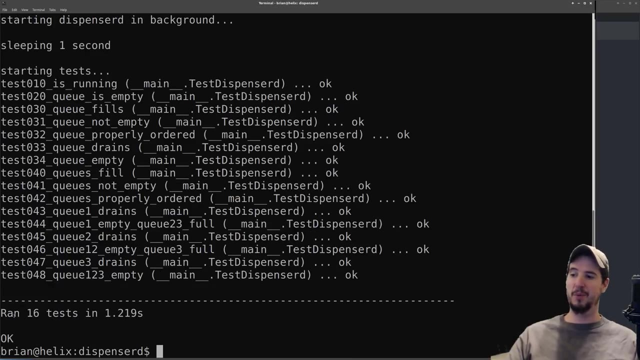 DispenserD, Just so you can quickly see how the tests work. once I'm in the folder, I have a script called run tests and then when I run that it will start DispenserD. It runs several tests and it'll let me know. it ran 16 tests and everything's okay. You could. 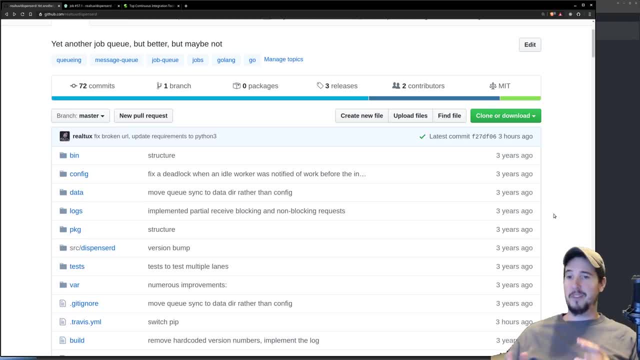 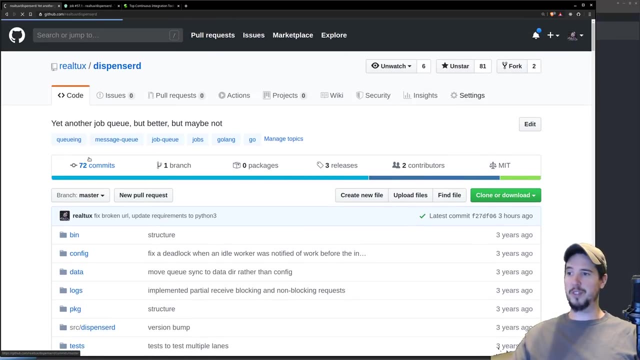 see that each test ended with an okay. Once I'm done with every test, I have my test. Really, my goal here is to make it so: every time a commit occurs onto this particular project, I want to automatically run those tests, And the way this works is: every time a commit occurs onto this Repository, it triggers. 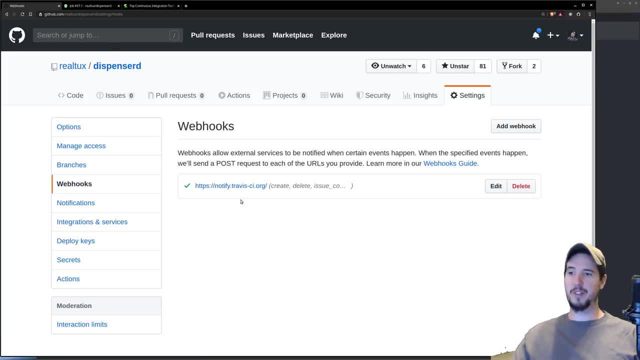 a webhook And if we go to webhooks here in GitHub, we can see that there is a webhook sending to notifyTravisCIorg. Once TravisCI receives notification that a new commit has occurred, the first thing it's going to do is spin up a virtual machine and it's going 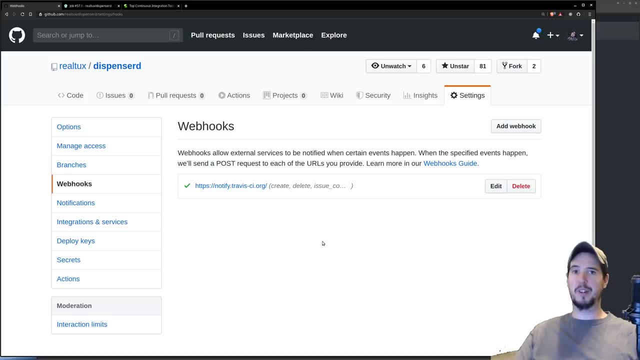 to actually clone the current test. So the first thing it's going to do is spin up a virtual machine and then it's going to actually clone the current test version of the repository to that virtual machine, in the case of travis ci, once it clones that. 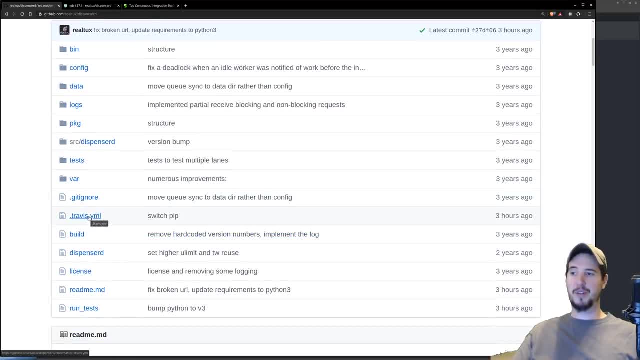 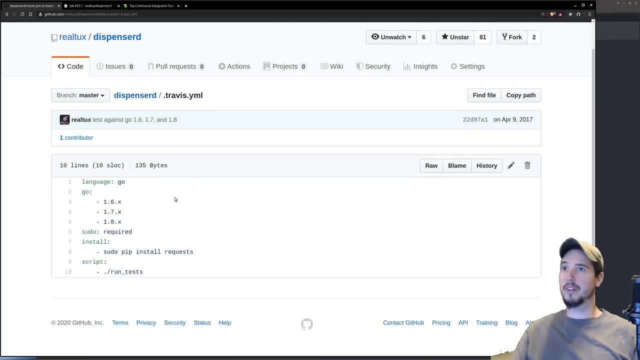 repository to the virtual machine. it's going to look for this file called travisyml, and it's this file that's going to be used to actually describe exactly how the continuous integration should work. now, while this configuration is specific to travis ci and the configuration 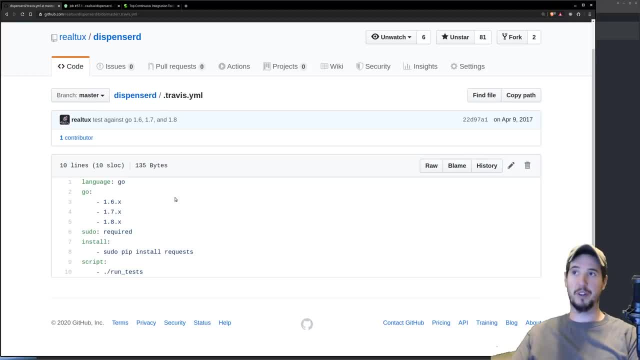 for another product is probably going to be different. the concepts of how this work are going to be mostly the same and, in this case, the things the continuous integration system needs to know about is: first, what language do you want to test? against which versions of that language? 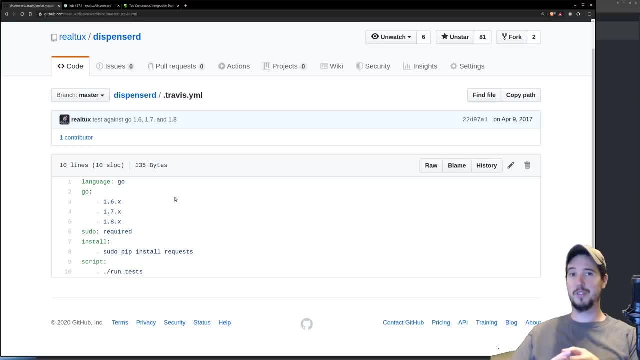 do you want to test against? what are the prerequisites that you should install prior to doing the testing, and then what's the actual script that you should run to run those tests? so first i'm saying the language is go and then i want to test against 1.6, 1.7, 1.8. keep in mind this. 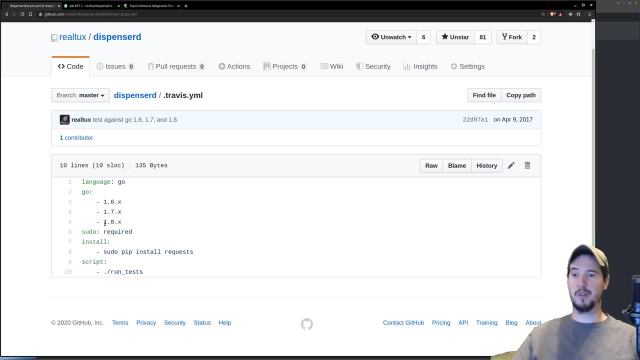 product is old. at the time, 1.8 was the newest version of go. of course, at the time of this video's recording. you know it's much newer, but that was the highest version at the time for the prerequisites. because my test file uses python requests to make http calls, i need to use pip to install requests. 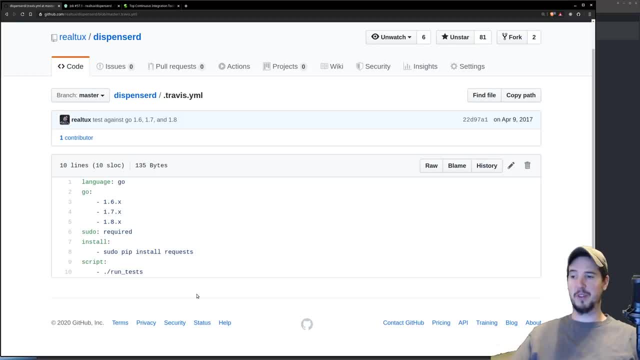 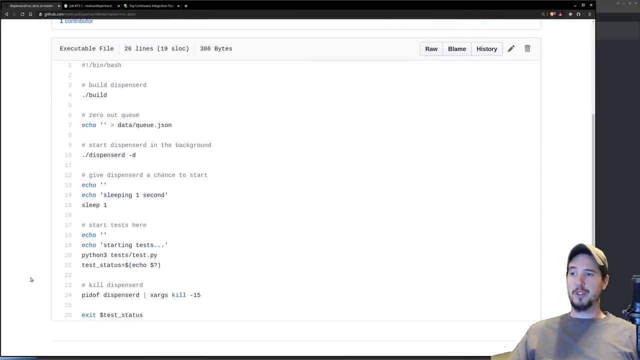 and find the script that should run when the continuous integration system starts up is going to be run tests and if you look at that file we can see that it has several things in it. don't worry too much if you don't understand exactly what you're reading here. there's really 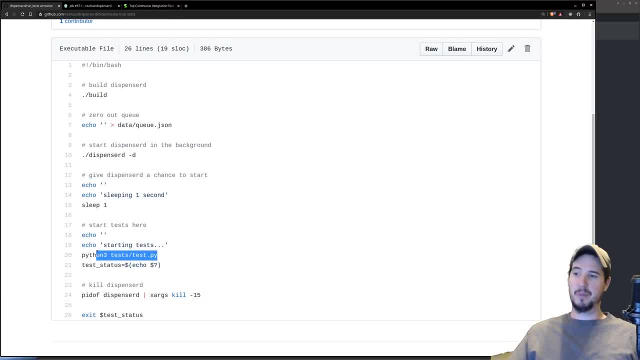 only three lines in this file that matter. the first is that python 3 runs my test file and then i store the resulting exit code in a variable called test status, and i do that because on line 26 i then need to basically exit this script with that specific status. the 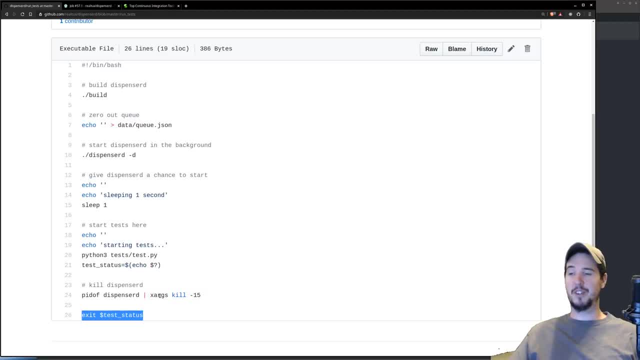 reason i have to do this is because travis ci is going to look at that exit code and that's how it's going to determine whether or not the test actually passed or failed. keep in mind that most continuous integration systems are language agnostic and they don't have any concept of 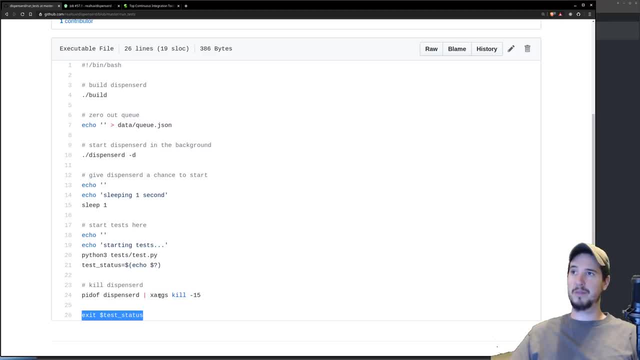 say python tests. they deal in exit codes. so if the exit code is zero, it's seen as a pass. if the exit code is non-zero, then it's seen as a failure. so now we have our webhook all set and we have our test ready and we have our configuration file done. let's go look at what it looks like on the travis. 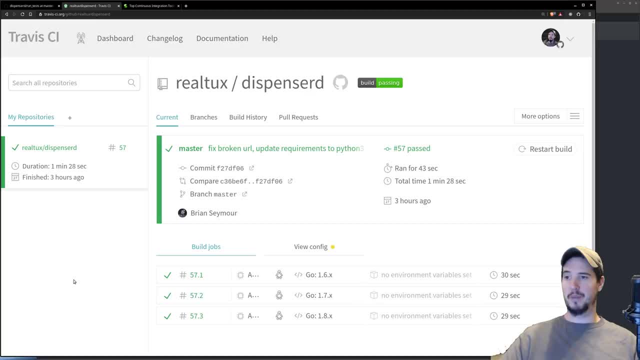 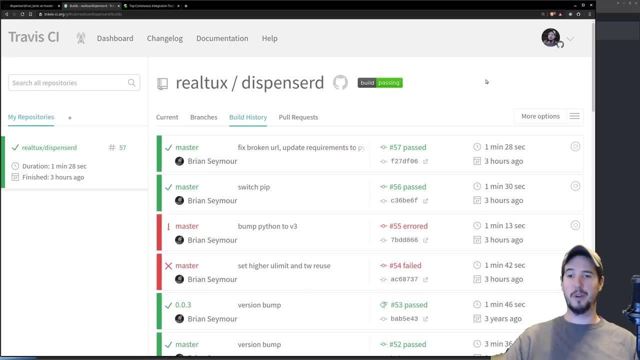 ci side on the dashboard for this project, it's going to show the most recent build and this is what you can see here, and this is one that was done about three hours ago. the other thing it'll show you is the entire history of every build that's ever done, and then its result, so green. 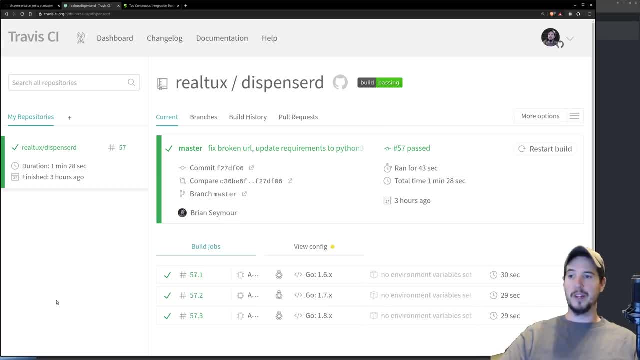 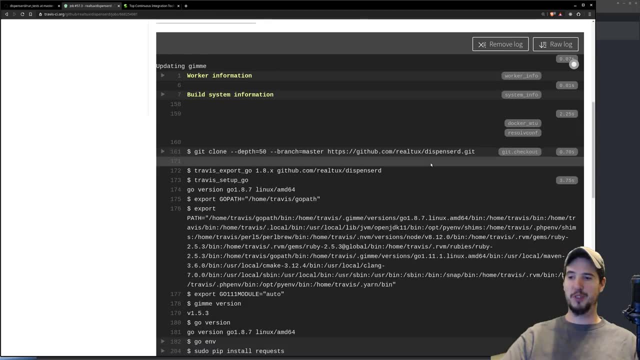 of course is it passed, and then red, of course is that it failed. but not only will the build show you the actual result of the test, it'll actually show you exactly what it ran. so if we click one of these here, we'll see a bunch of terminal output. 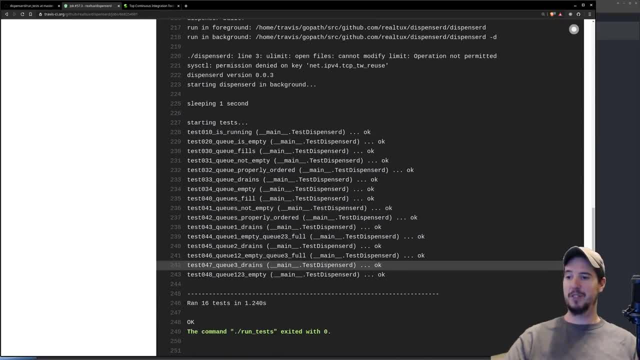 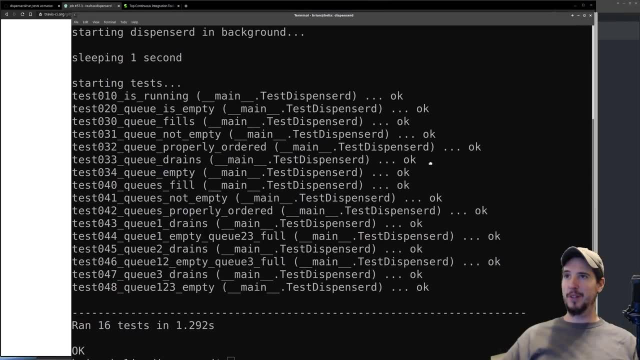 so what we're actually seeing here is the result of our tests, and at the bottom you can see the command run test exited with zero. now you may have noticed that the output here is the exact same as the output that was in our terminal earlier when we ran them manually, and that's because it's 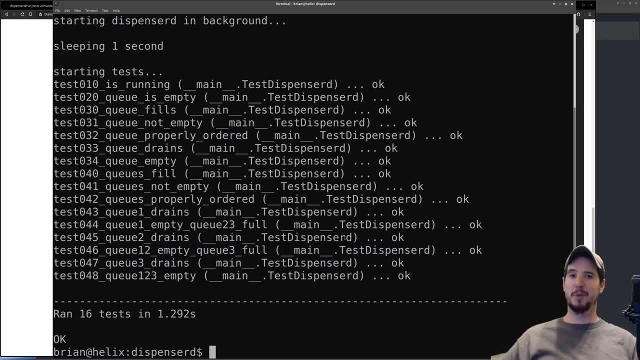 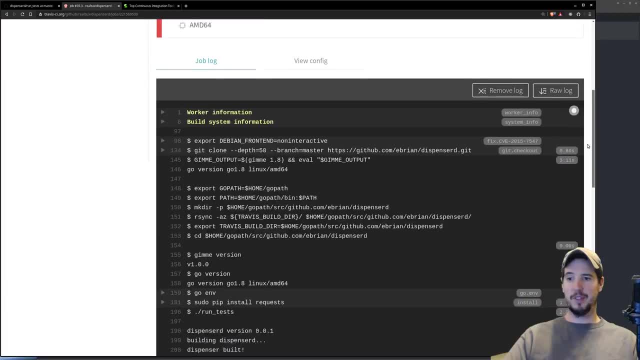 running the exact same script in pretty much the exact same environment. you know, but it's doing it automated. now, just for contrast, i want to show you what a fail to test would look like. so in this case, if you remember how all of them used to be okay, you could see that the first five were okay. 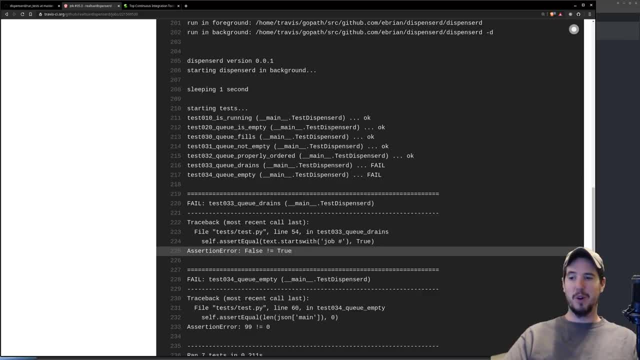 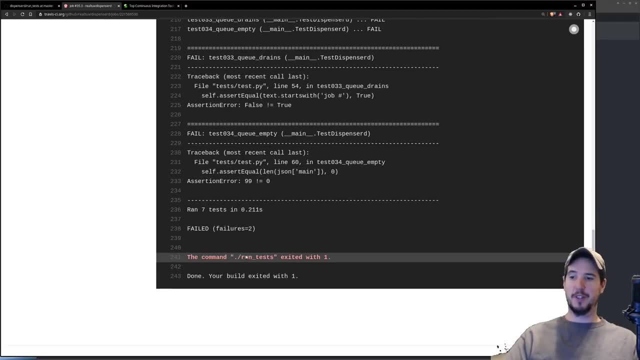 and then the last two were failures and it actually states here exactly why the failure was: false is not equal true. and then you look at the test and you can see exactly why that was. and at the bottom here you can see where it says: the command run test exited with one. so because it was non-zero. 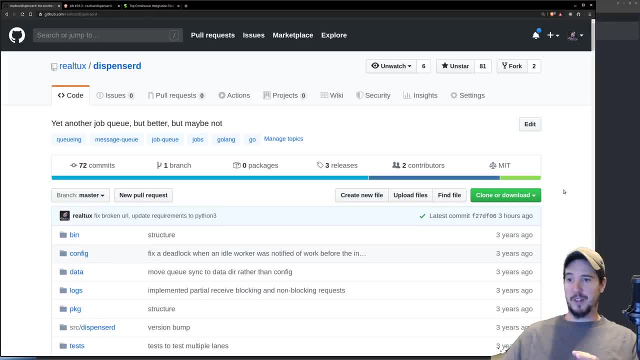 travis ci treated that as a failure. so the final result here is that we have our project, we have a test suite and then we have an automated system that makes it so: anytime there's a commit to this project, it automatically runs those tests against those changes to make sure everything still works.